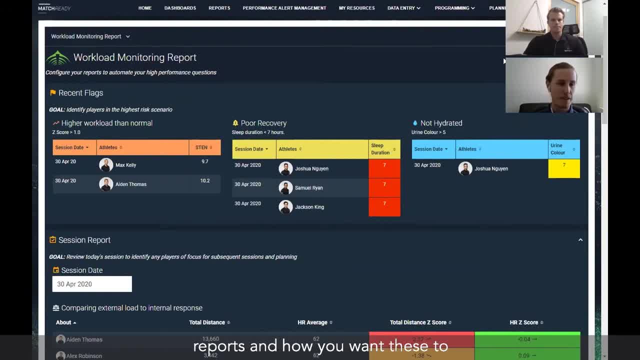 to determine the complexity of these reports and how we want these to look, With these as well. on top of that, we're essentially trying to tell a story with this visualization, to influence the program in an actionable way. We don't want to just present. 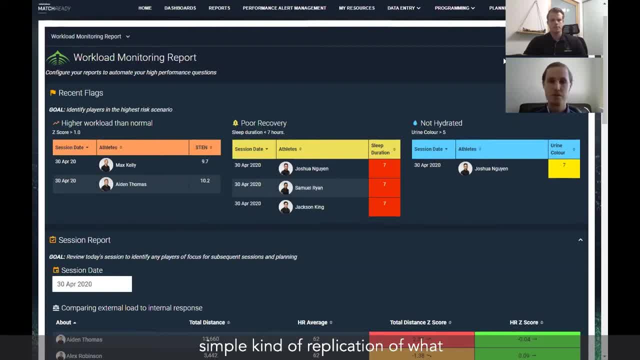 the data in a simple kind of replication of what the session elicited. We want to know what that means in reference to where we've come from with this athlete and where we're going to go tomorrow or, say, leading into a final series or a championship, whatever that might be. 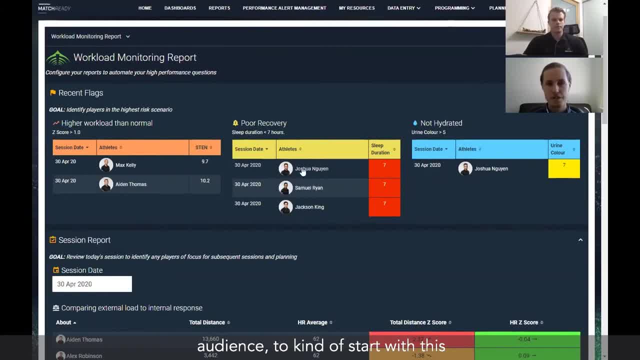 And then I guess, in terms of the audience- to kind of start with this report- we've got a lot of coaches and practitioners all over the world that just want very simple information. They want that alert, They want to land in the platform and see the most recent flags, And then they want to go. 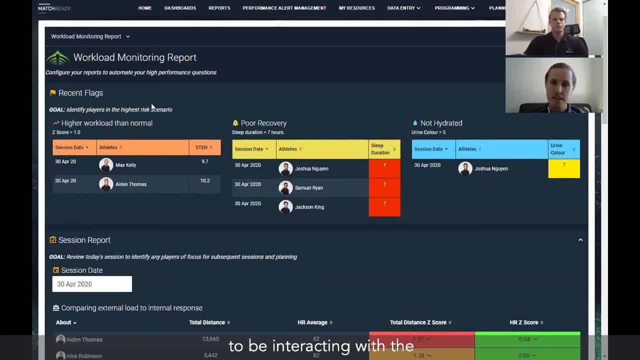 they want to be out of the AMS and they want to be interacting with the athletes and actually having those discussions. So the very kind of simple layout I've got here is for those practitioners that just want to get in and out. I've just got my most recent flags. 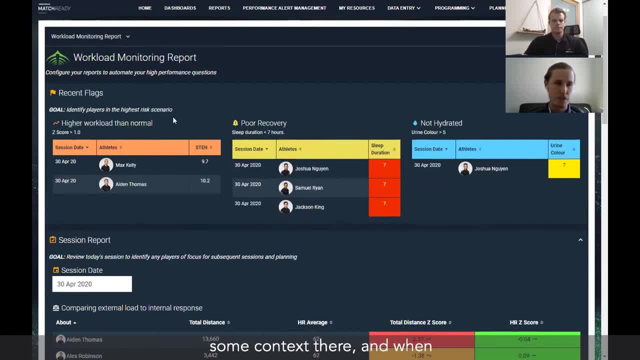 I've kind of put a goal across each of these visuals to kind of give you some context there, And we're looking at whether we can identify the highest risk scenarios or athletes in the highest risk scenario. So examples here: we might have a higher workload than normal. This is using that Z. 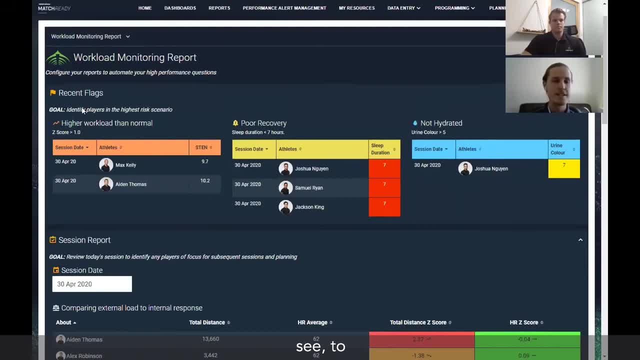 score converted to a STEN here, as you can see, to identify if someone's above their average or significantly above their average load, So I can quickly maybe interact with that player and actually have them do an additional recovery session or, you know, do a little bit of a. 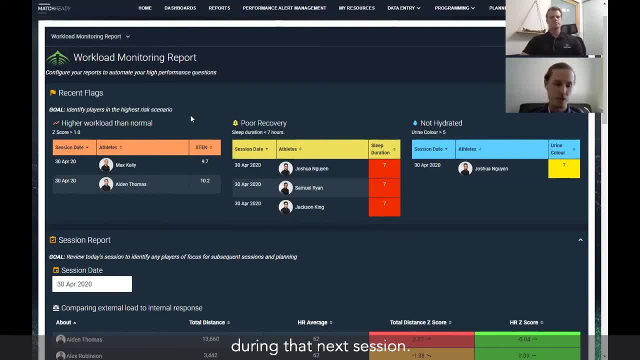 get in some additional warmup drills during that next session. I could have some recovery related or even internal response metrics coming through from my various wearable devices, or even a self report questionnaire via our mobile application, and identify if there's any players that potentially haven't got that adequate recovery that we want throughout the program. Again,